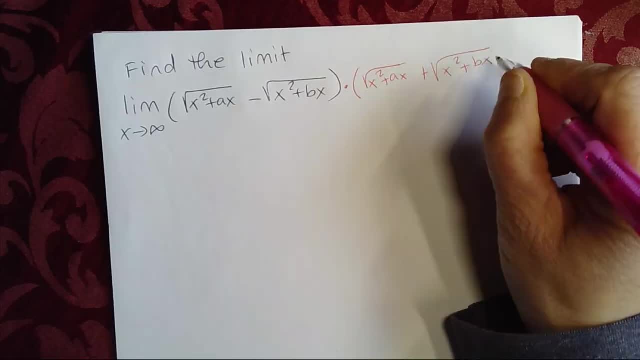 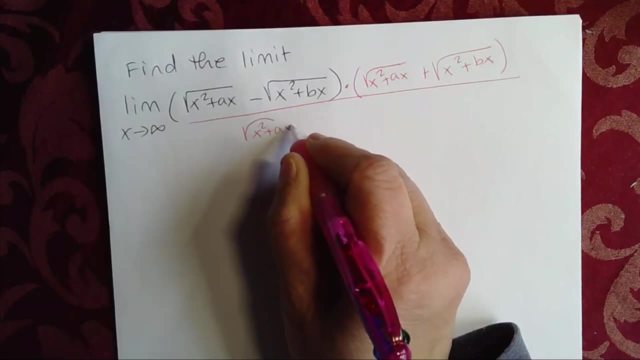 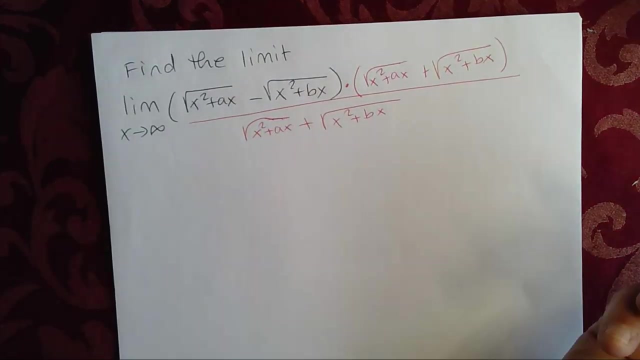 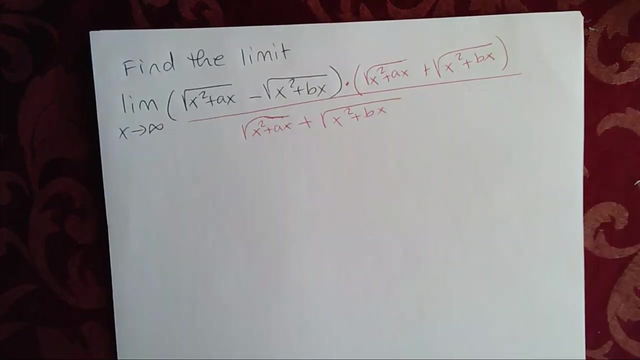 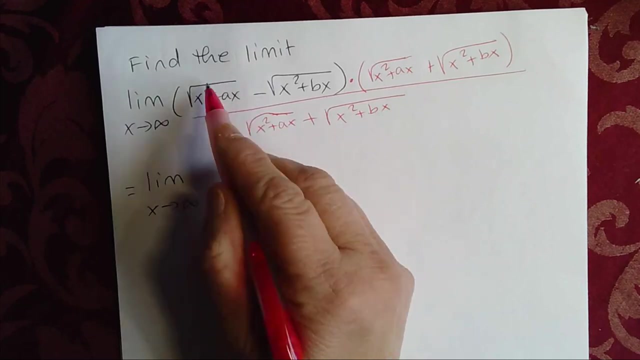 of x squared plus bx, both the numerator and the denominator. Remember, we are multiplying by 1 plus square root of x squared plus bx. Now, when you multiply these two, you're multiplying the difference and sum of two. So this is equal to the limit as x approaches infinity, of this one squared, so this is square. 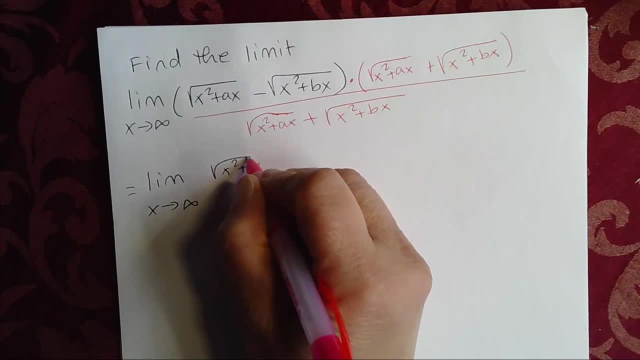 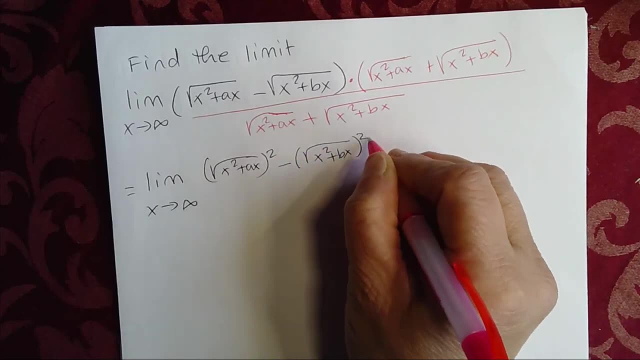 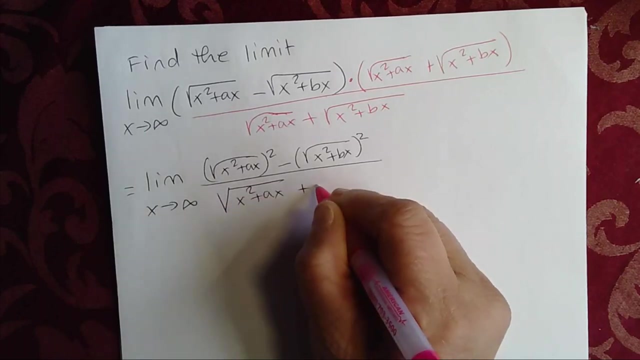 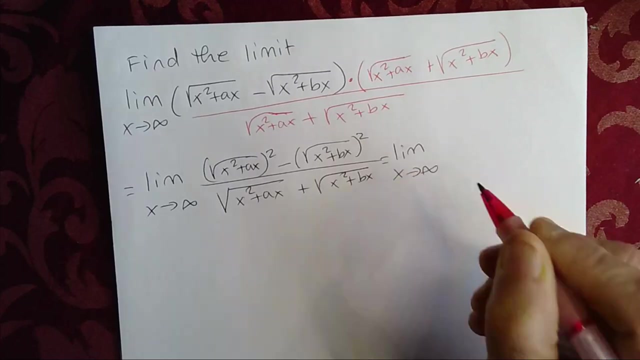 root of x squared plus ax squared minus the second term squared, so x squared plus bx squared divided by the denominator, So x squared plus ax plus square root of x squared plus bx, And this is equal to the limit. as x approaches infinity, The square cancels the square root. 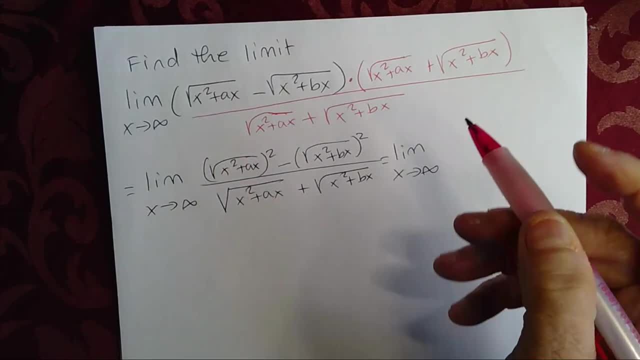 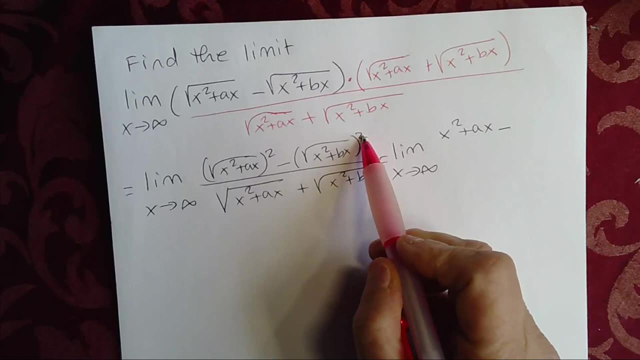 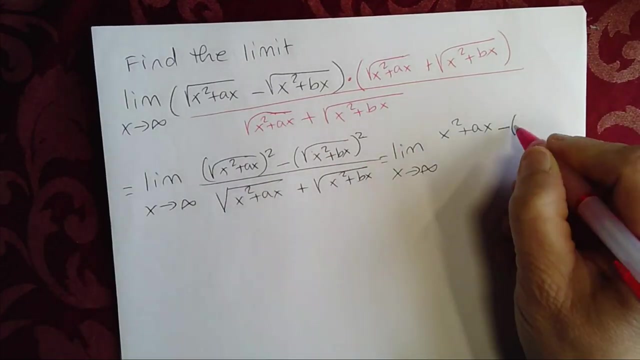 What comes out is the radicand, So that's equal to x squared plus ax minus. same thing here. the square cancels the square root. What comes out is x squared plus bx. But be careful, we need to put parentheses. You have a minus here, So that's x squared plus bx. 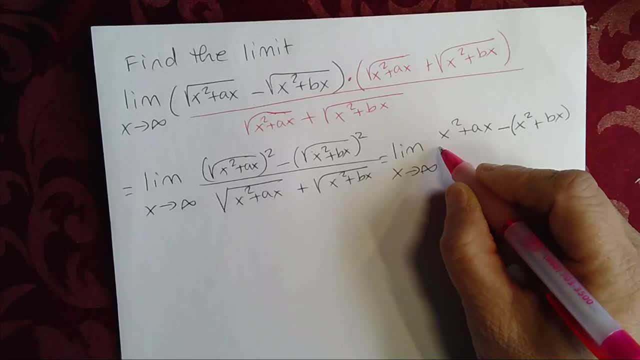 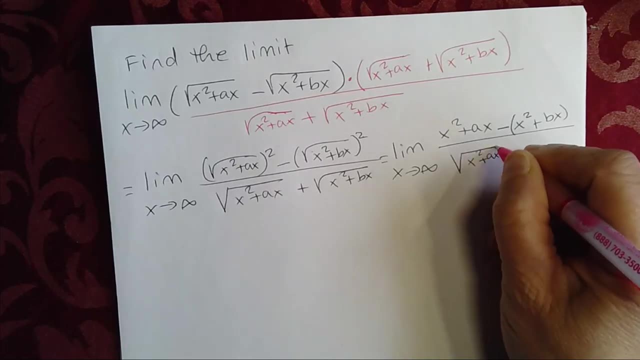 You may want to put parentheses here as well. It's up to you. It's not me. I'm going to give you a plus, But you have that option: x squared plus ax plus square root of x squared plus bx. You notice, here you have x squared And if you distribute the negative, you're going. 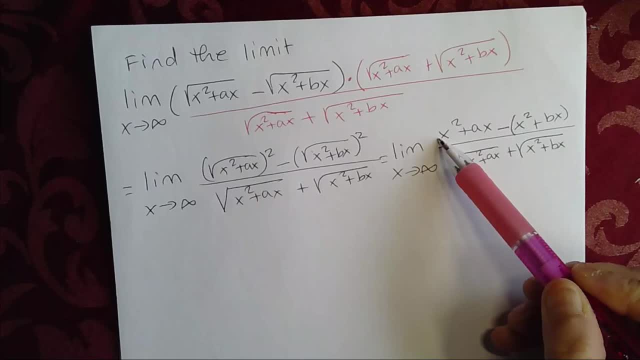 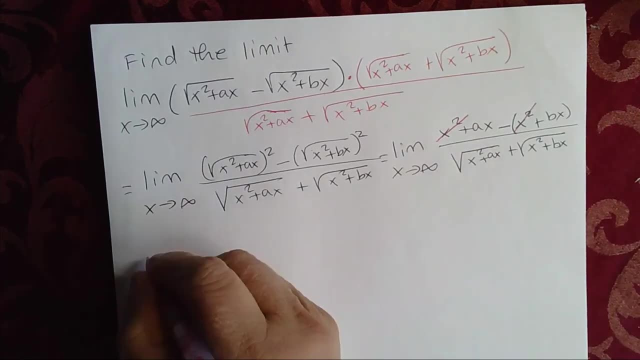 to get negative x squared, So you can cancel these out if you like. So let's do that. The x squared cancel with this x squared And what you're left with that's a limit as x approaches infinity. So you have ax minus. 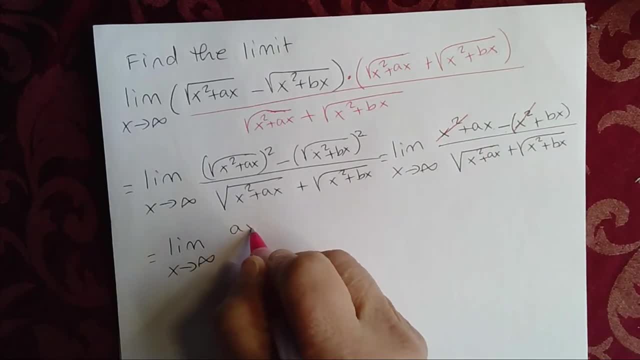 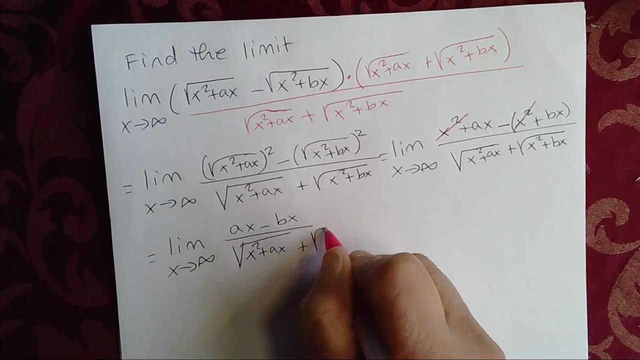 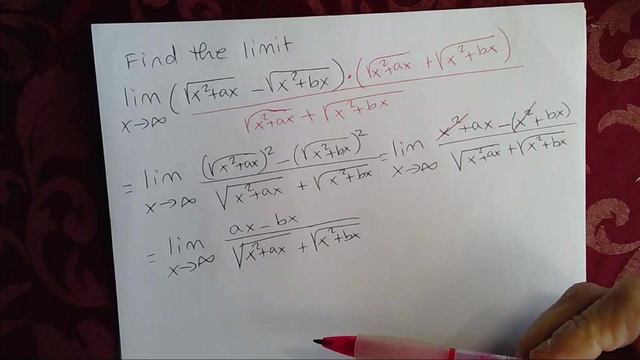 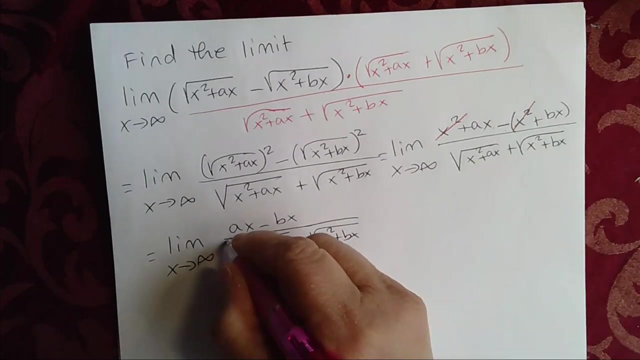 bx divided by square root of x squared plus ax, plus square root of x squared plus bx, now the variable with the highest power in the denominator hits the square root of x squared. so what you do here, you can go ahead and divide this one by here, by square root of x squared. now, before we're going, 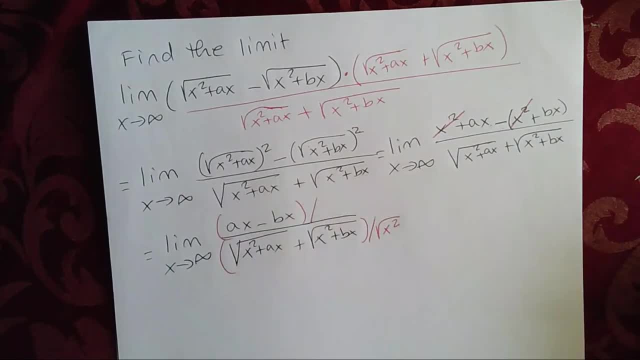 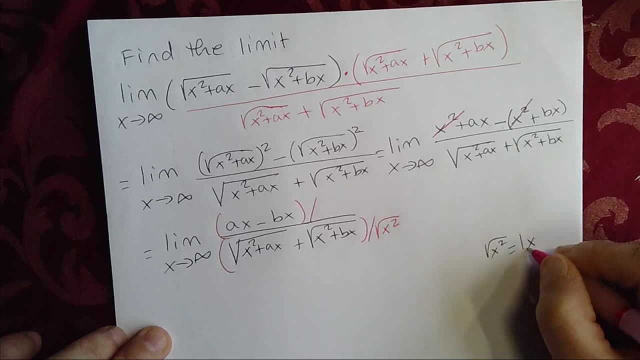 to do the same thing here. you can divide here by square root of x squared as well, or you can do it directly. what is square root of x squared? square root of x squared is the absolute value of x. well, x, in this case is approaches infinity. so x is positive. so that means this is equal to x. 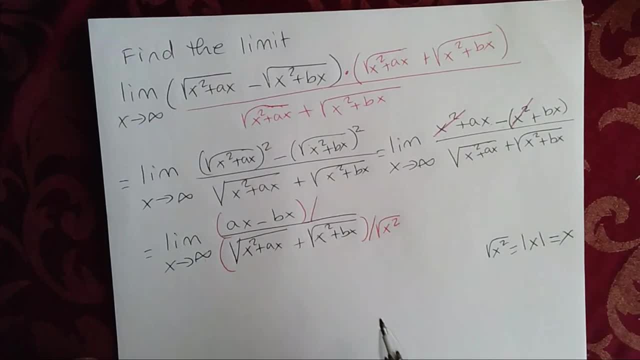 so you can, if you want to here, divide by square root of x squared, like we did here, or square root of x, squared in this case, is also equal to x. you may want to divide by x as well. either way would work. this will help me simplify the next step. that's why I did that. so now this is equal to the limit. 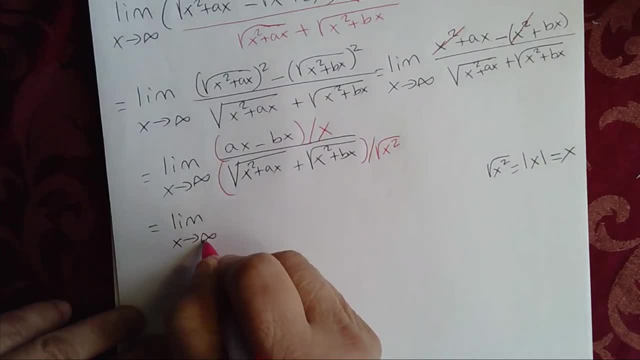 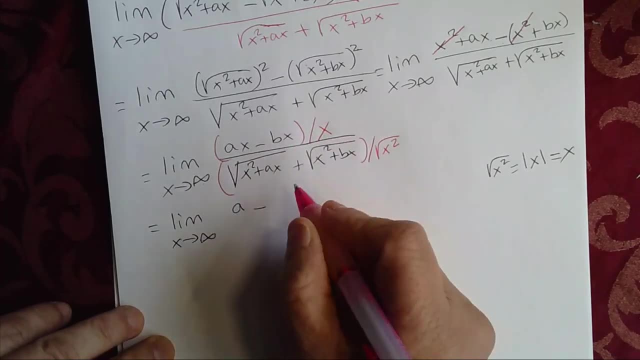 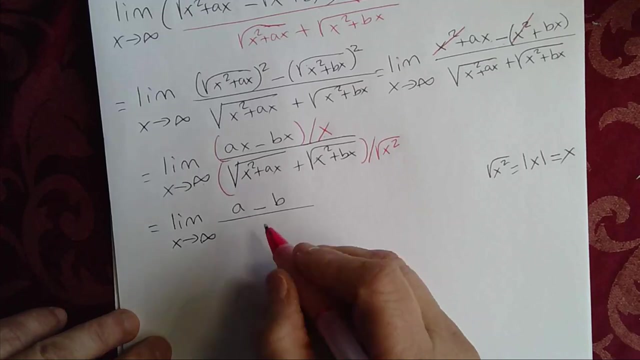 as x approaches infinity. ax divided by x, that's a minus bx divided by x, that's B divided by. you can take the x square inside the radicand or you can simplify directly. it's up to you. I'm going to go ahead and take it inside the radicand. 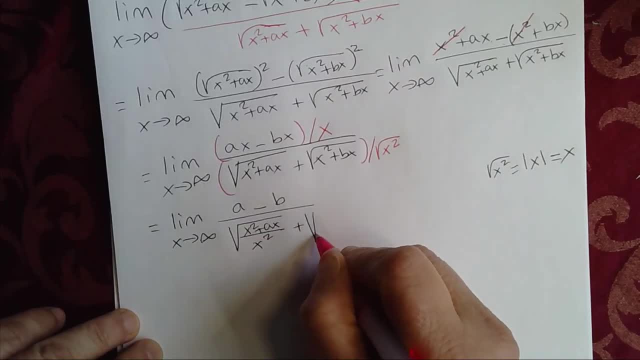 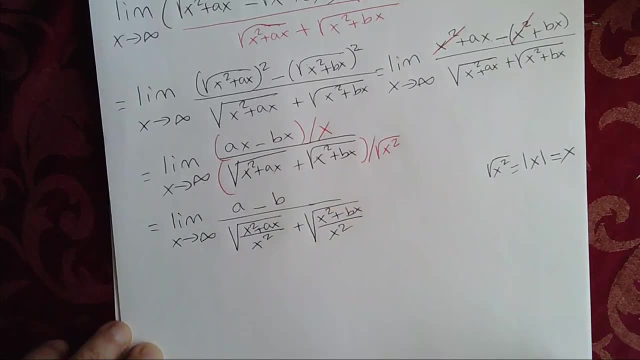 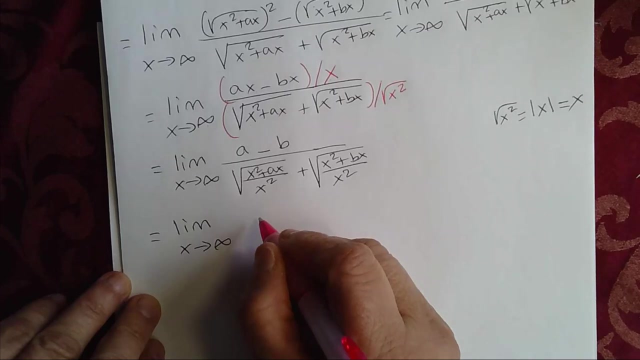 so that's square root of x plus bx divided by x square. and simplifying this, what do we get? that's equal to the limit, as x approaches infinity, of a minus b divided by square root of x squared. divided by x squared, that's one plus ax. divided by x squared, that's a over x. one of the x's cancels. 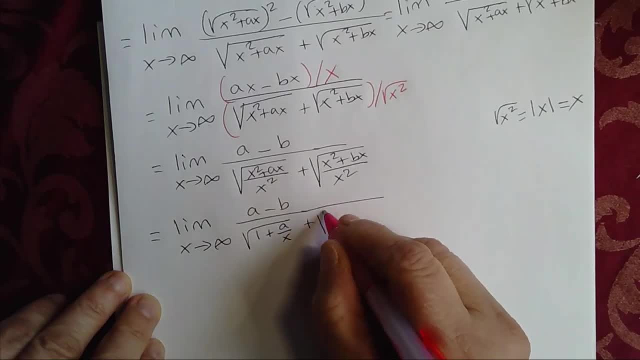 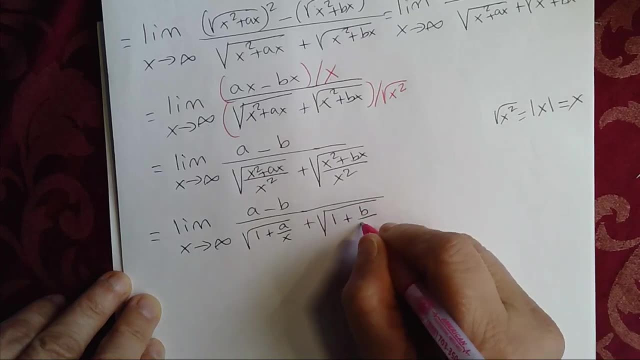 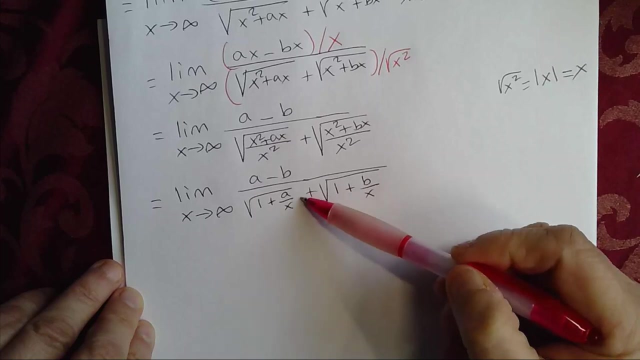 plus square root of x squared divided by x squared, that's one plus bx divided by x squared, that's b over x. now, as x approaches infinity, a over x approaches zero. so remember, x approaches infinity, a over x approaches zero and also b over x approaches zero. remember you are dividing a number, a and b by a. 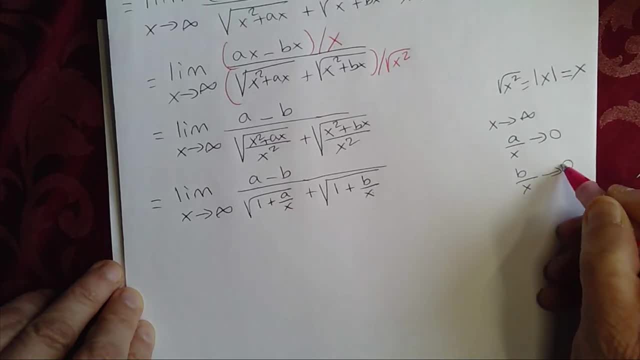 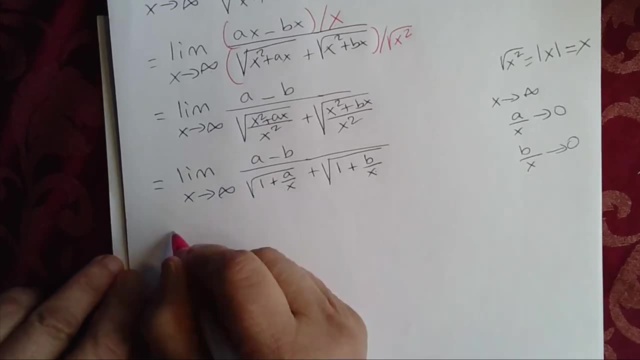 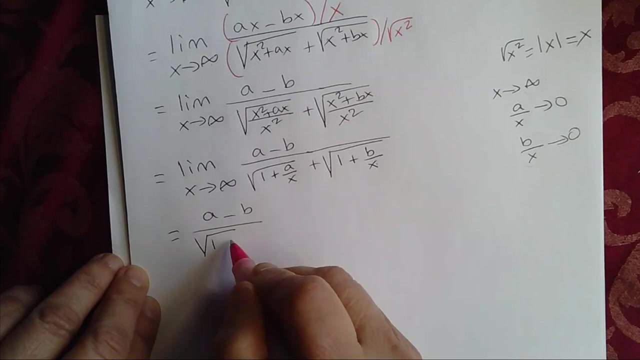 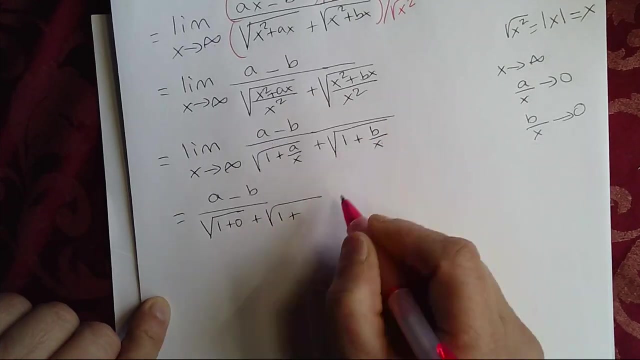 very, very large number, a number that's approaching infinity. so the fraction approaches zero. so this is: this becomes equal to a minus b divided by square root of one. this is approaching zero. so plus zero plus square root of one, plus this becomes zero as well. so that's equal to a minus.